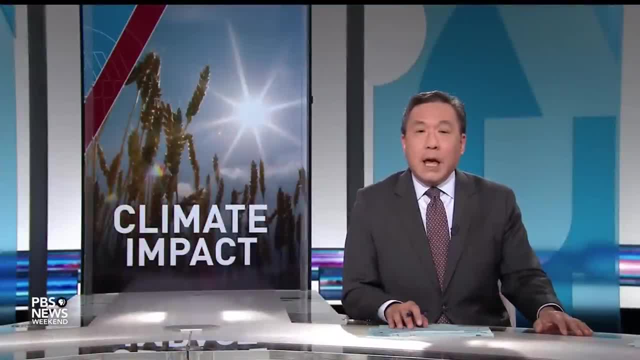 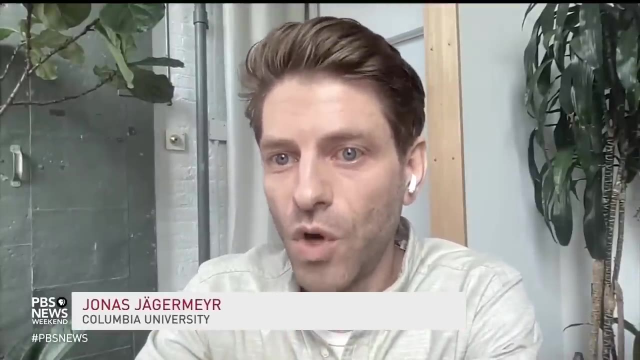 Earlier, I spoke with Jonas Jagermeier, a climate change scientist at Columbia University and the NASA Goddard Institute for Space Studies. I asked him to explain the relationship between climate change and the global food supply, If you're asking for the main drivers, factors that really affect crop growth in the field. 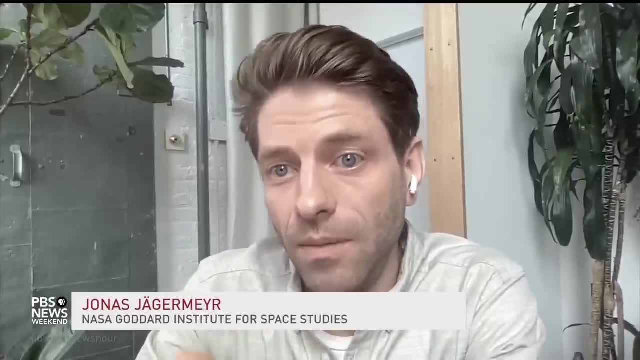 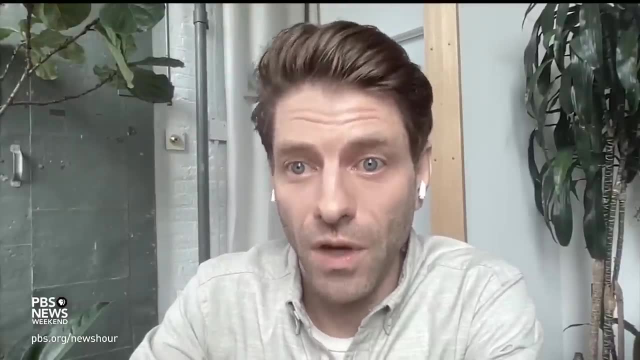 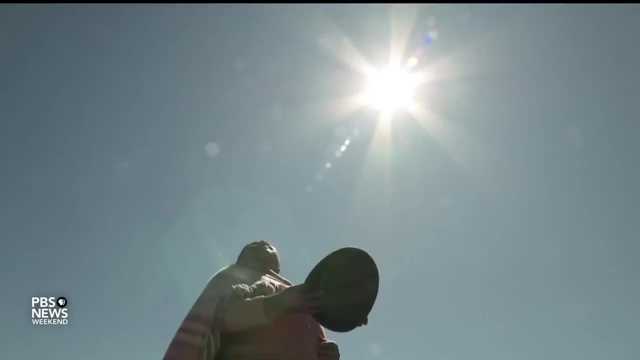 then it's mainly three aspects: It's temperature, it's precipitation and then something that's much less known is carbon dioxide, CO2, in the air. You know, in temperature and precipitation they create extreme events such as droughts, heat waves, and then hail and flooding is. 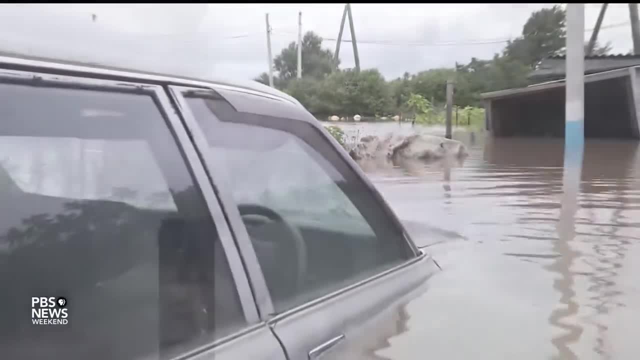 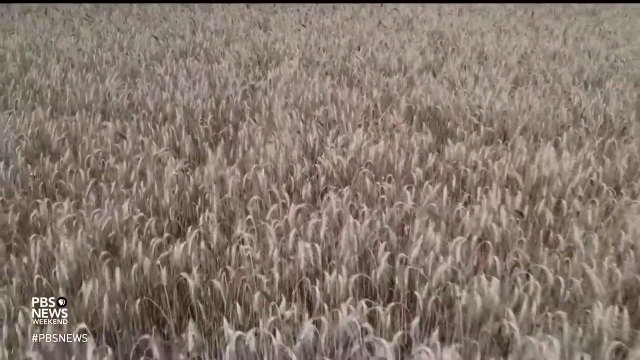 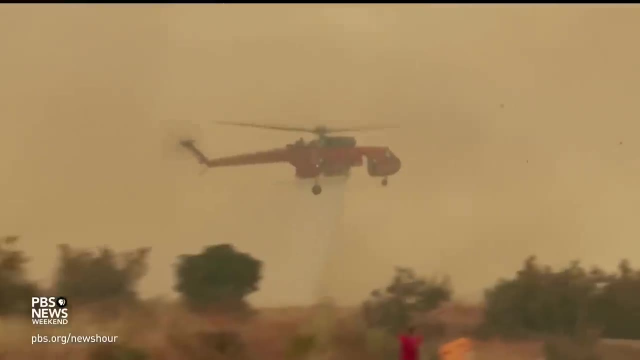 in the air. There's a big problem in agriculture too. But the CO2 effect it creates climate change, if you will. At the same time, crops love it. The plant growth is stimulated by CO2.. At the same time, it creates adverse effects. through all these paths, getting effect from. 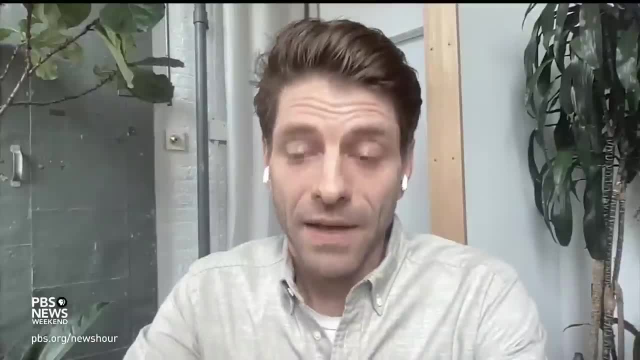 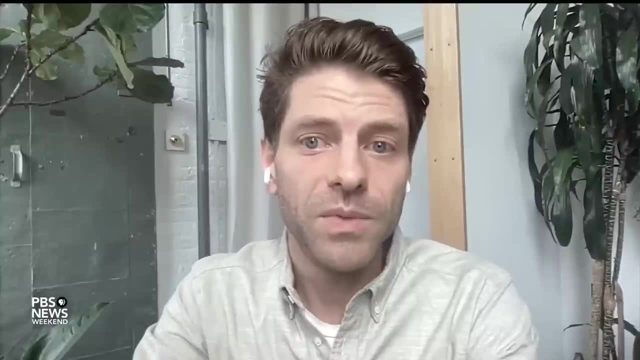 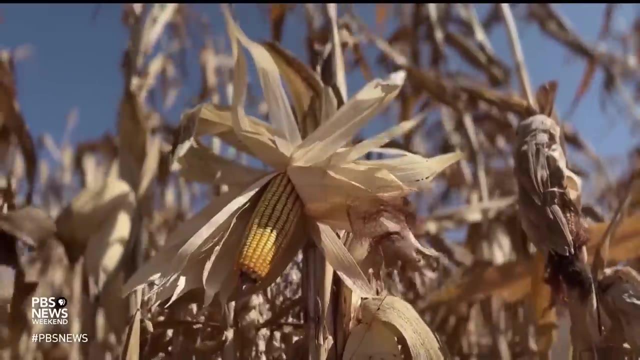 climate change. Does this affect all crops the same? That's a very good question. Some crops are very sensitive to that CO2 effect. Other crops are not. So, for example, corn maize doesn't really benefit from higher CO2 levels, So the full brunt of temperature. 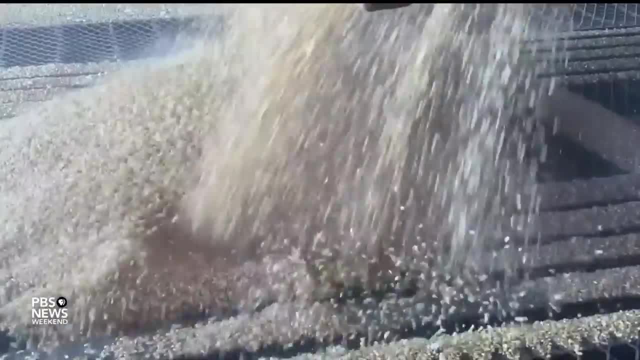 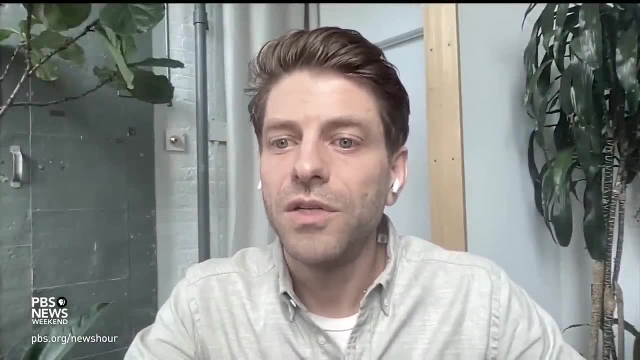 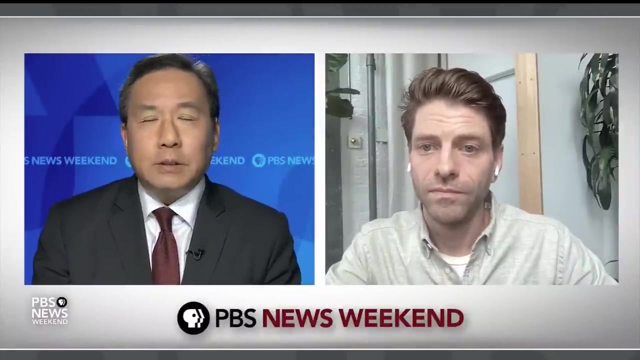 and shifting precipitation patterns are felt in maize growing, So globally aggregated corn is really seeing the largest negative impact. So it sounds like they're winners and losers in terms of crops and in terms of regions. I think that's a message that 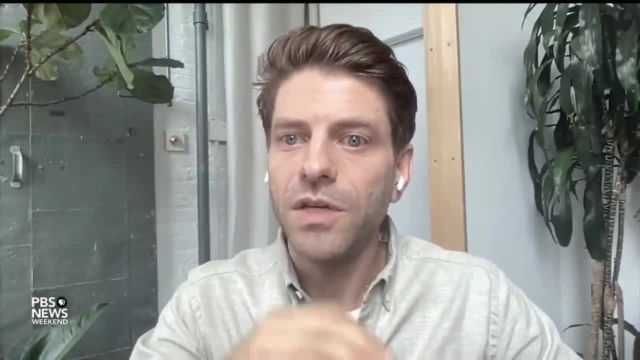 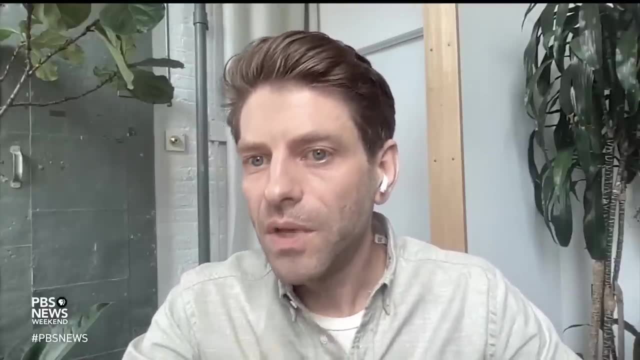 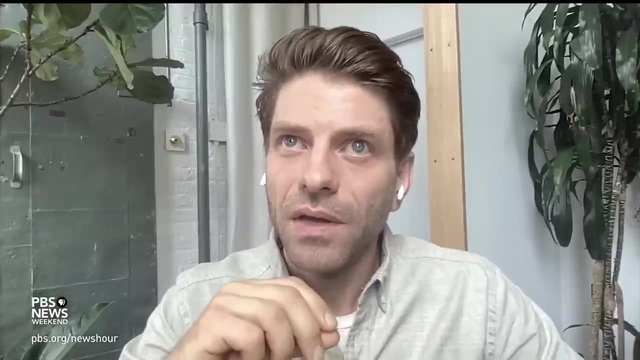 we need to get comfortable with, And it does mean that climate change isn't just a negative blanket of adverse impacts. But we want to be really careful because potential positive or potential gains are difficult to realize And what's important is to think of the regions where they could. 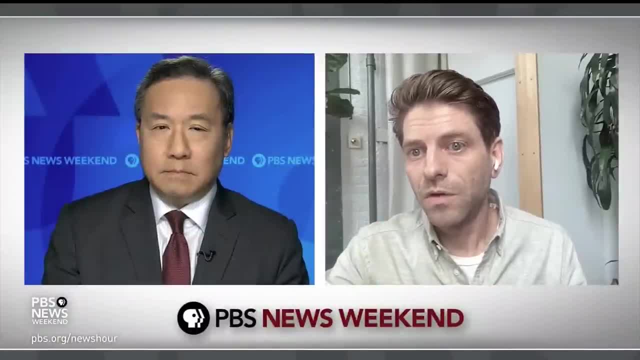 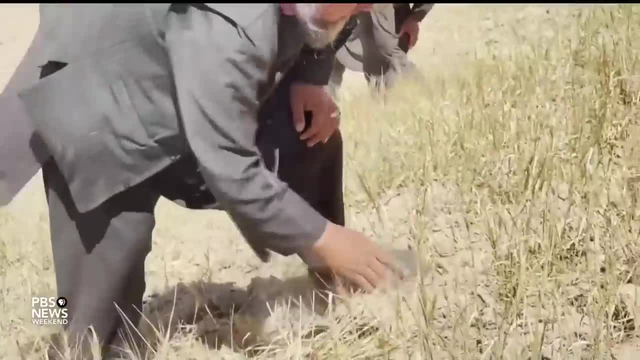 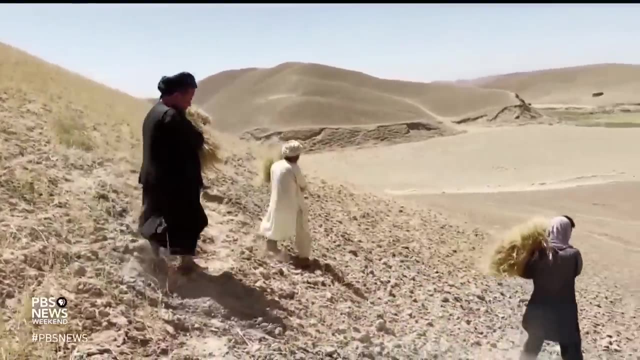 happen. So low latitude. generally we're speaking of lower-income countries, small land farming that have much less capacity to adapt. So large countries say yes, but small countries say no. Small- afective problems also While or negative impacts will directly impact livelihoods and the food system in general. 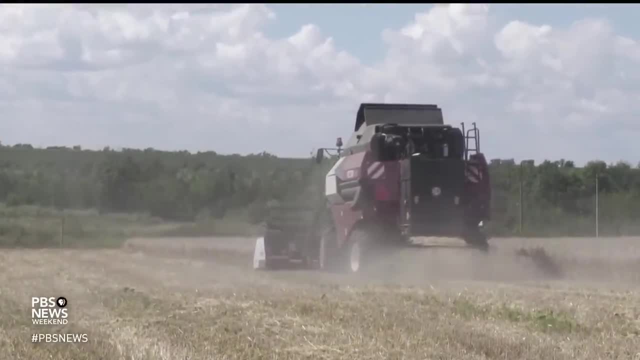 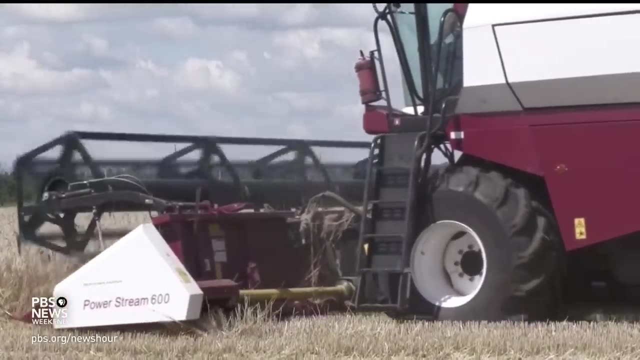 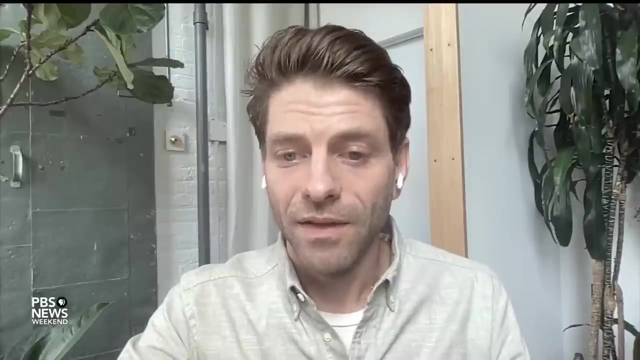 Whereas in developed breadbasket regions in the global north there's more adaptation capacity that can buffer some of these negative impacts, And this can also affect the nutrients, the nutritional value of crops. Is that right Correct When I say CO2 is beneficial for plant? 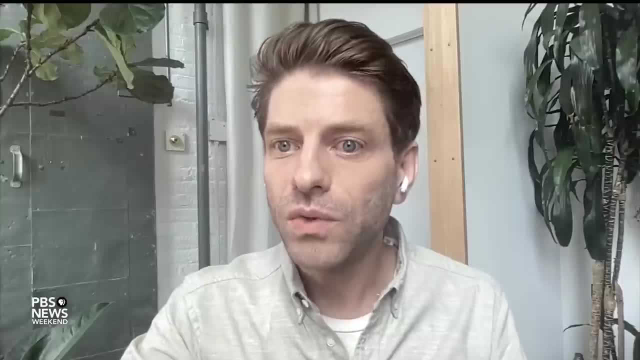 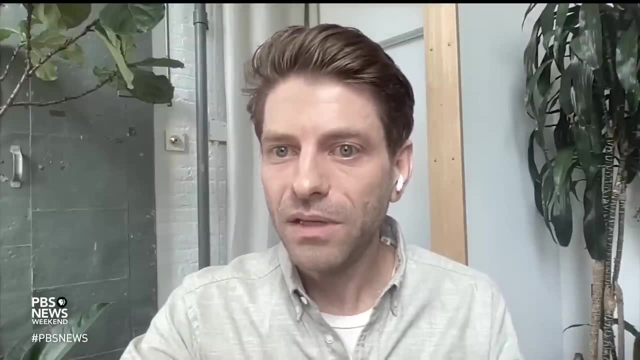 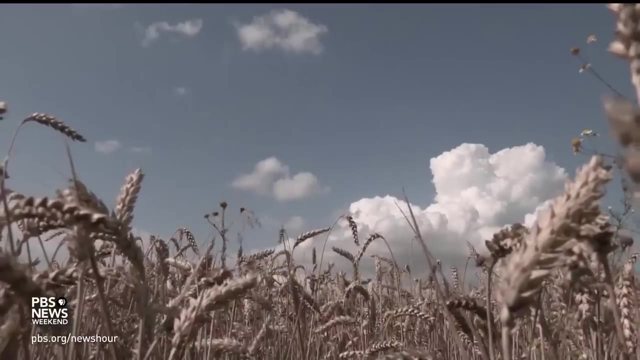 growth and development. at the same time, it dilutes the nutritional content of crops, So it moderates any gains you may see from higher CO2 levels and the nutritional quality: the protein content, micronutrients such as zinc, and vitamins and iron. 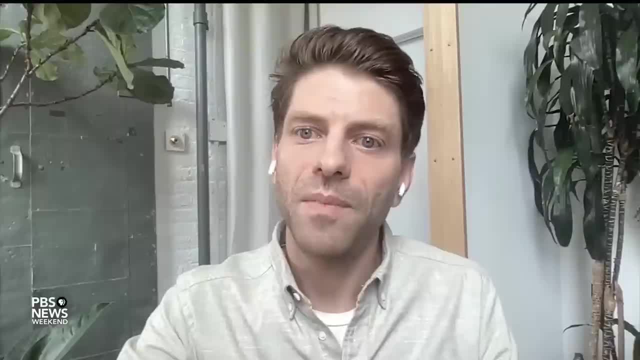 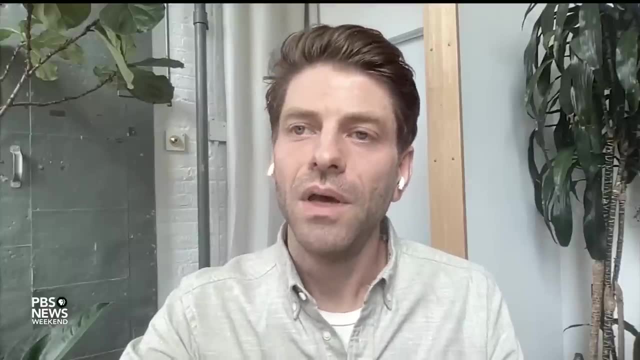 These components aren't taken up, aren't produced by the crop at the same pace they're growing. They're not taken up, aren't produced by the crop at the same pace they're growing. So it's a dilution effect and it lowers the nutritional quality of the crop. 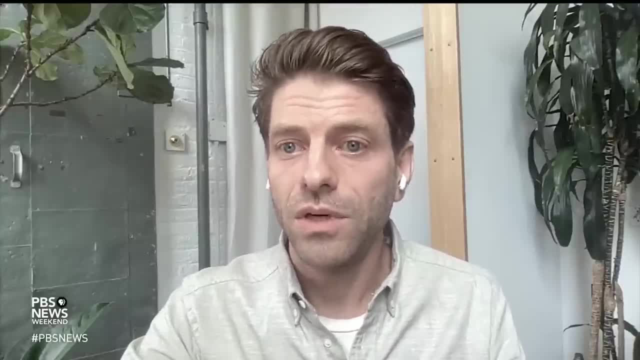 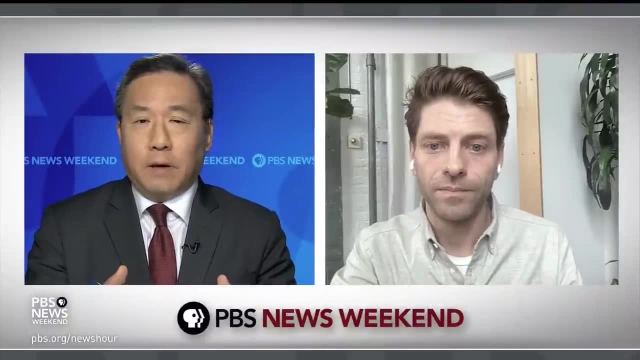 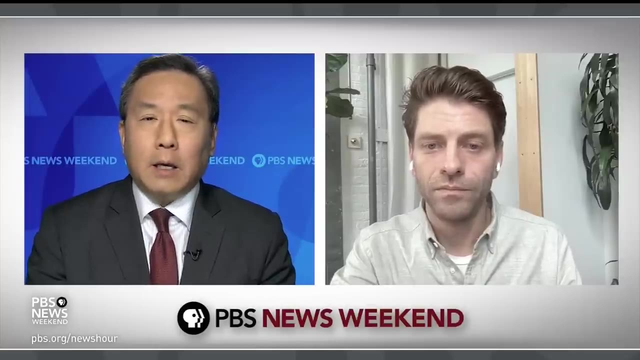 which raises concern for our global nutrition. Put this all together for us and tell us the practical effects of all of what you've just explained in terms of people's diets, in terms of food insecurity, in nations and in places that are already experiencing food insecurity. What? 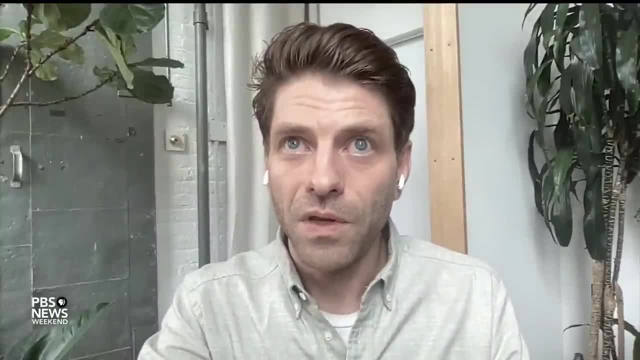 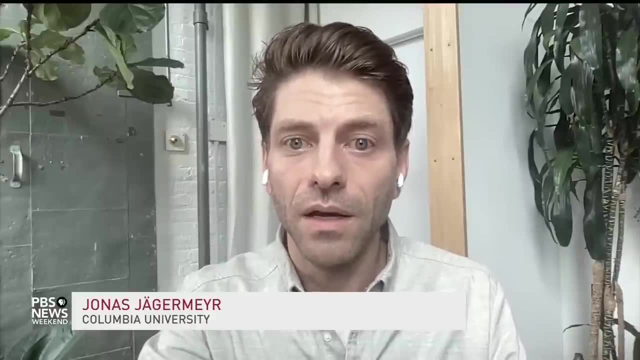 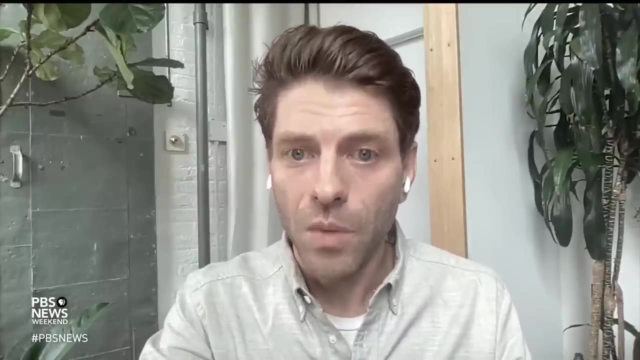 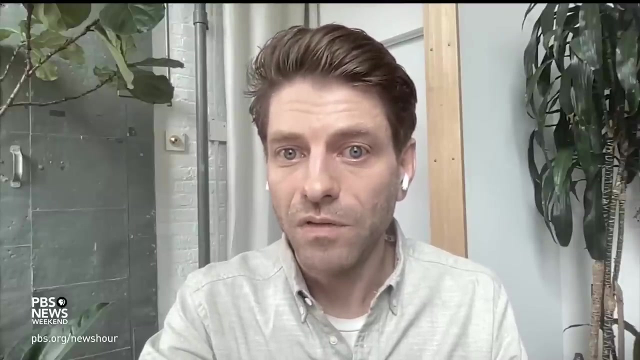 are the practical effects of all this. We have to get comfortable with the idea that agriculture is facing a new climatic realities and has to undergo a fundamental transformation. There will be winners and losers. Some regions may potentially benefit from moderate warming and higher CO2 levels. The vast majority of global best bread baskets will see adverse impacts And 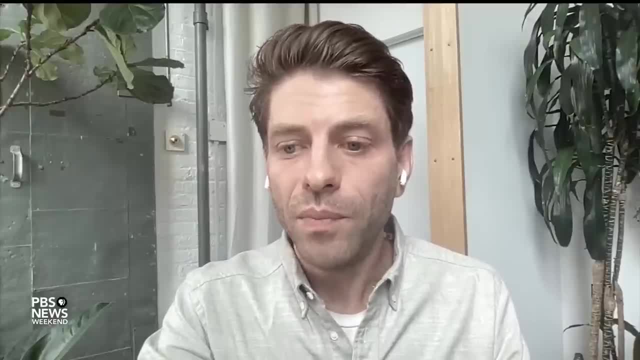 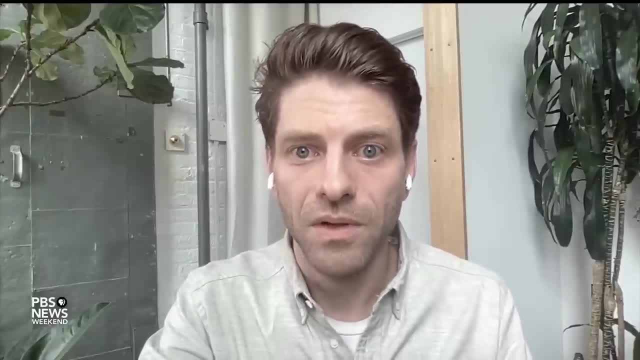 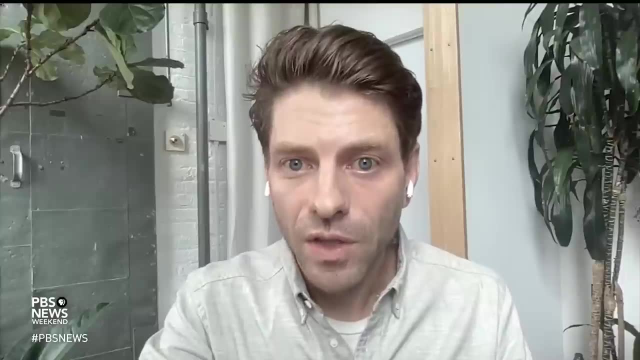 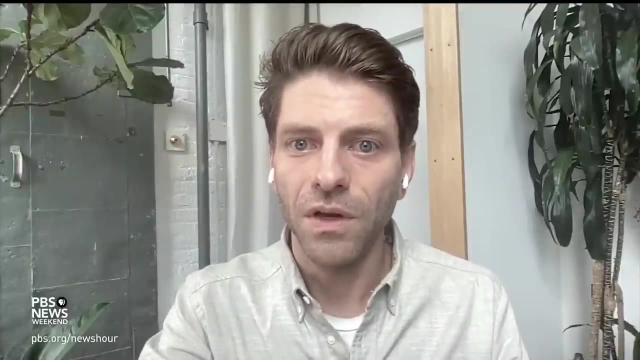 Proactive and long-planned adaptation implementation: That's the key to making global food systems sustainable and climate resilient. Adaptation: what needs to be adapted? The farmer in the field, first of all, can do intuitive things, such as shifting your planting dates If it's warmer.